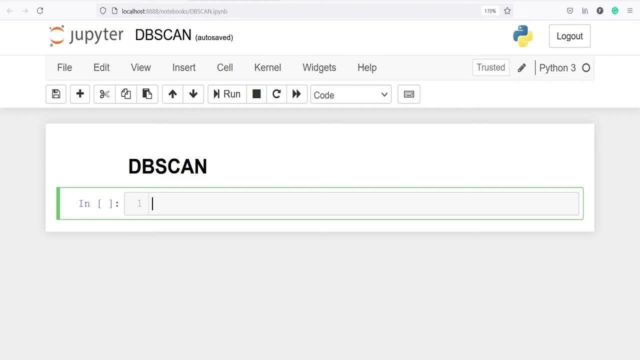 In this video, you will learn about dbScan algorithm in Python. dbScan stands for density-based spatial clustering of applications with noise. There are two important parameters in dbScan. The first one is minimum points and the second is epsilon. Epsilon is the distance around each object and minimum points are the number of points that must exist within epsilon distance from the point. 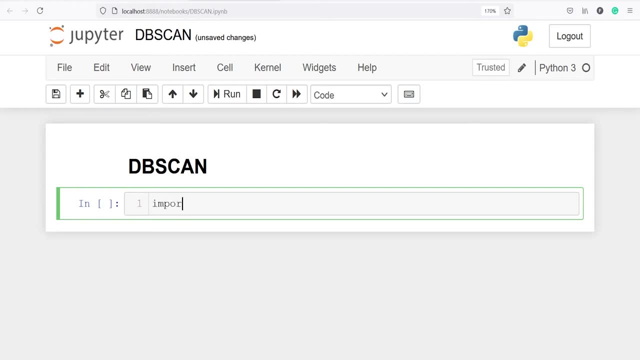 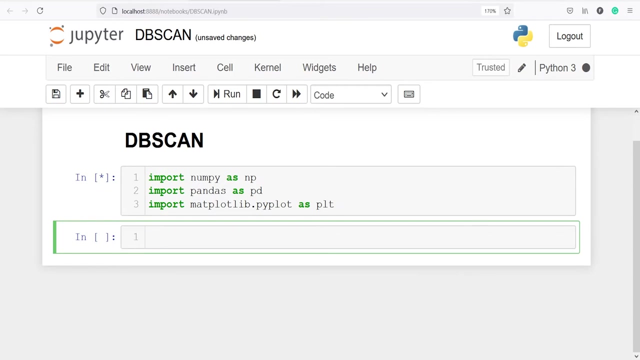 Let's import numpy as np. Let's import pandas as pd. Let's import matplotlib. import matplotlibpyplot as plt. We are going to work on the mall customers dataset. I'll show you the dataset now. This is the dataset. We have variables such as customer ID. 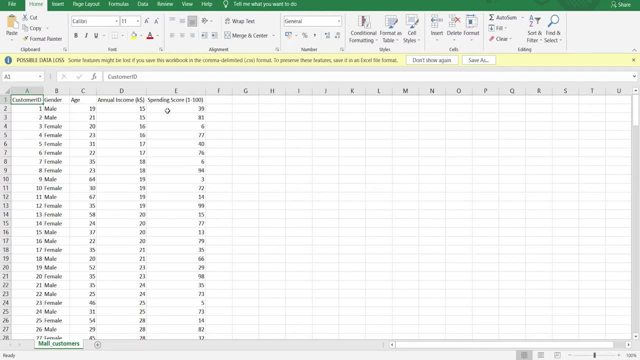 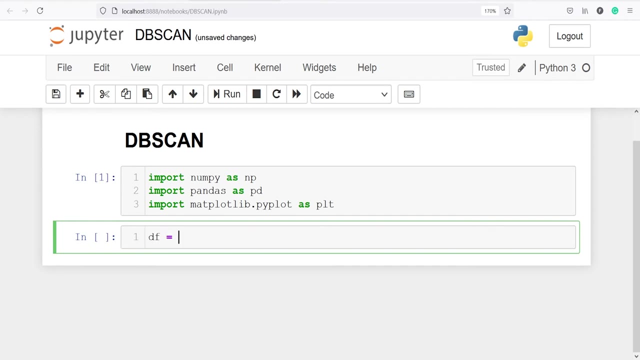 gender, age, annual income in thousand and spending score. We are interested in two variables: annual income and spending cost. So we are going to work on these two variables only. Let's make one variable, df. In this I will save the data frame. 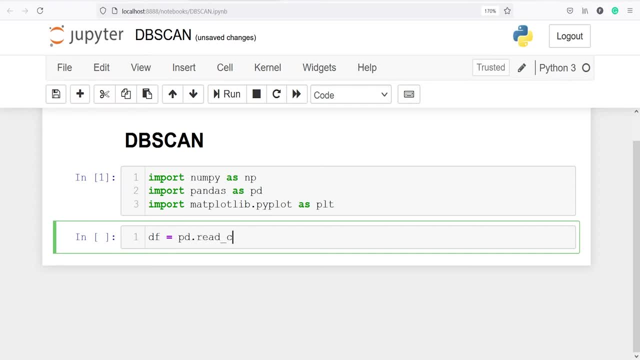 From pandas. I will call the method read: underscore csv. Inside this I will pass my csv file name and my csv file name is mall underscore customers dot csv. Let's execute our code. Let's look at the top five rows of our data frame df. 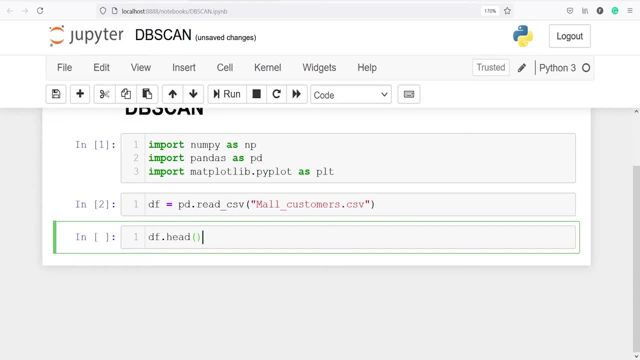 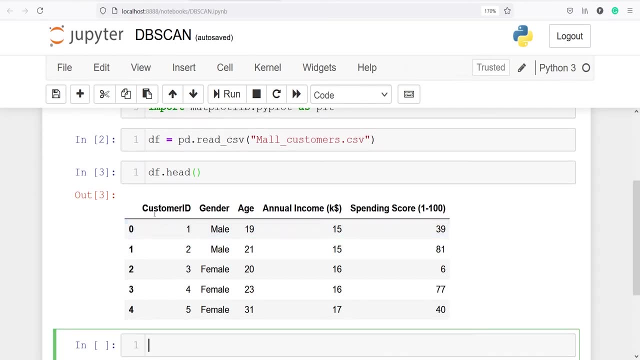 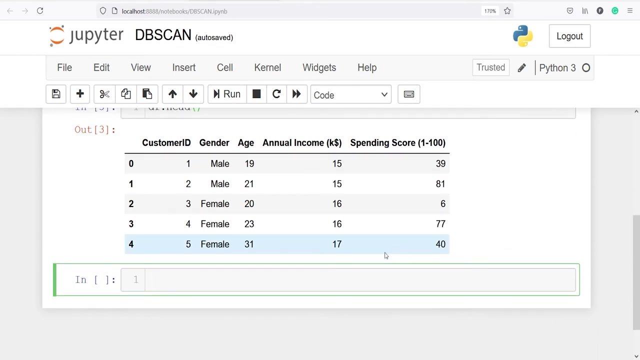 I will call the data frame df dot head. In the output we can see we got the top five rows of our data frame And we have variables such as customer ID, gender, age, annual income and spending score. We can also look at the bottom five rows of our data frame. 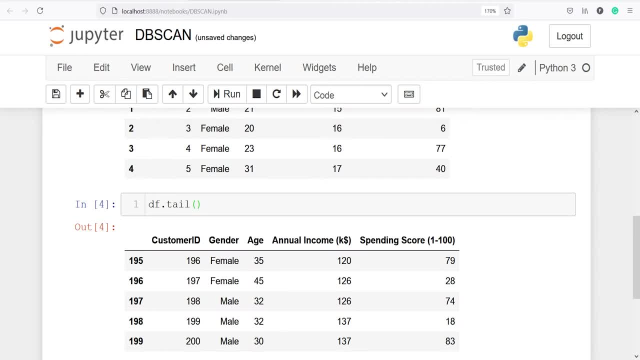 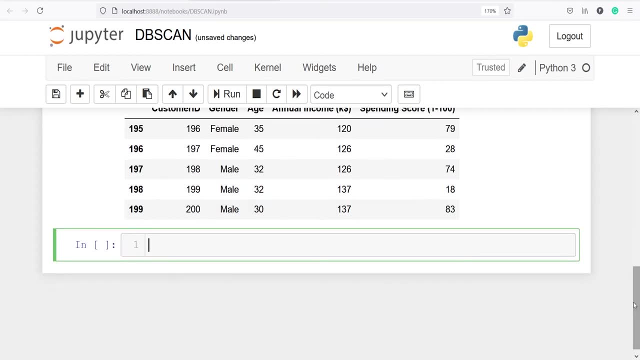 We will write df dot tail. These are the bottom five rows of our data frame, starting from 195 up to 199.. We can also check the shape of our data frame. We will type df dot shape. Shape tells us the number of rows and columns. 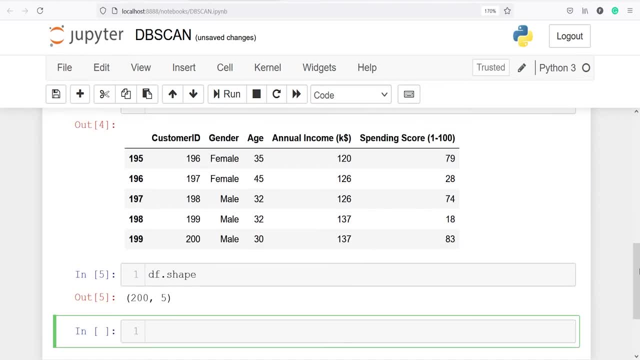 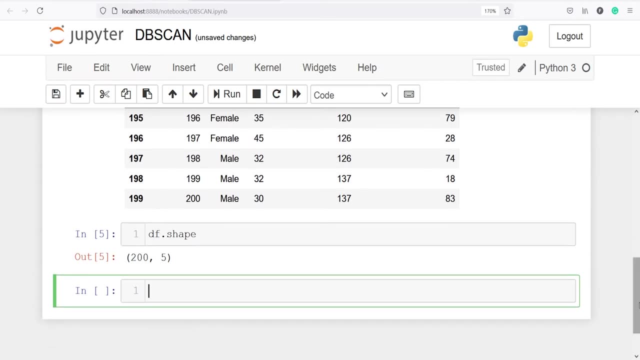 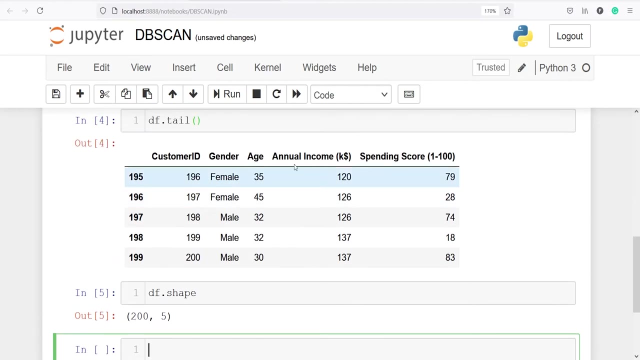 So there are total 200 rows and five columns. You can see all the five columns here: One, two, three, four and five. Now we will work on two variables: The annual income and the spending score, And the index number of these two variables are 0,, 1,, 2,, 3 and 4.. 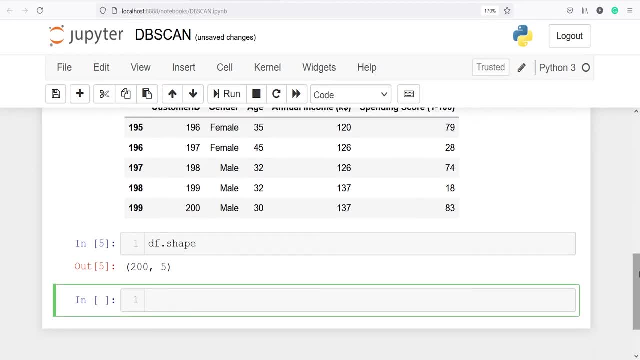 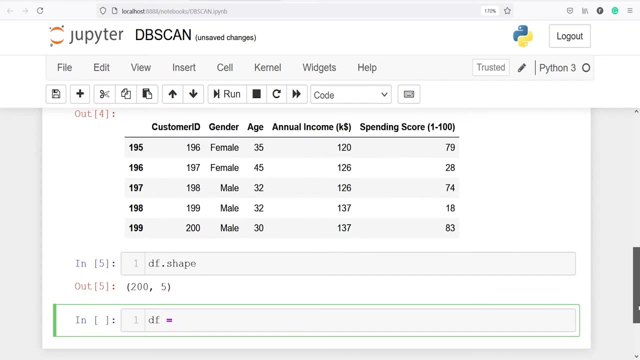 So the index numbers are 3 and 4.. Now I will make one variable, df, Because we are going to save one new data frame And that data frame will consist of only these two variables. Then I will call df, dot, iloc. 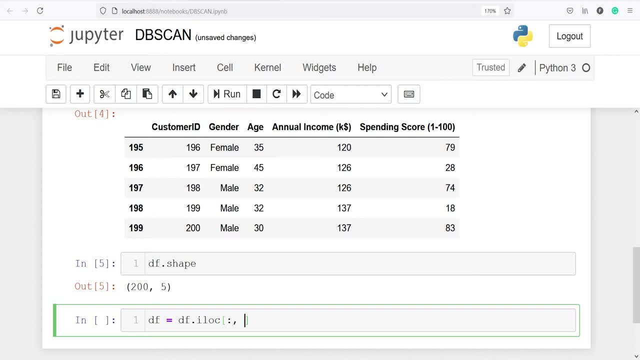 Inside this I want all the rows And I want only two columns. These two columns And the index numbers are 3 and 4.. So I will make a list And inside this I will pass the index number 3, dot 4.. 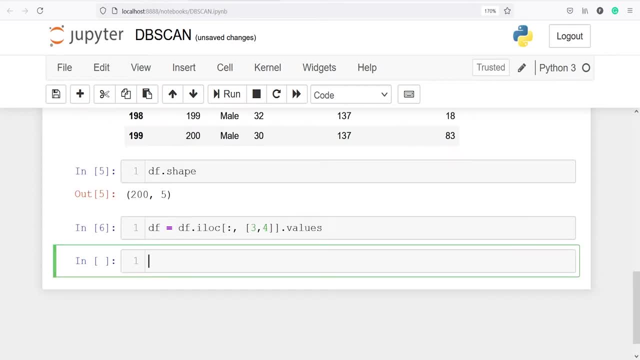 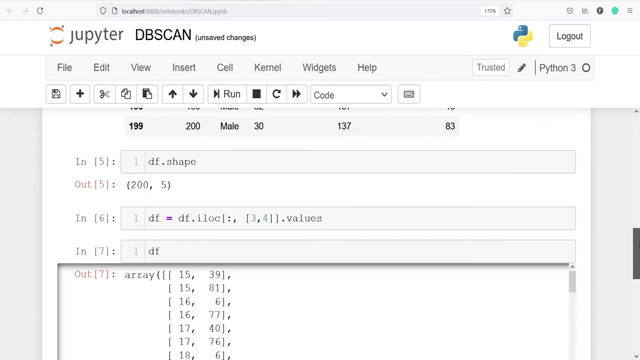 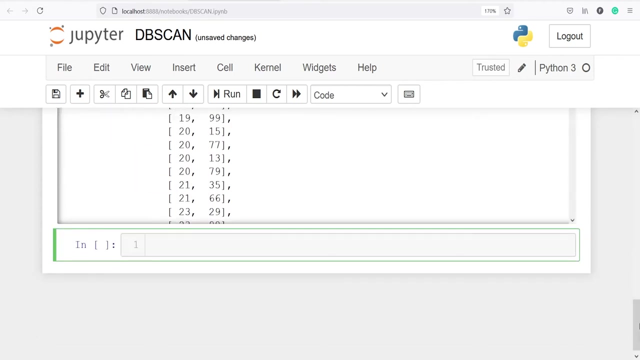 And then here dot values. I will type df And these are the values, Because we have only two columns now, And the two columns are this annual income and spending score. Let's visualize these two columns. I am going to plot it. 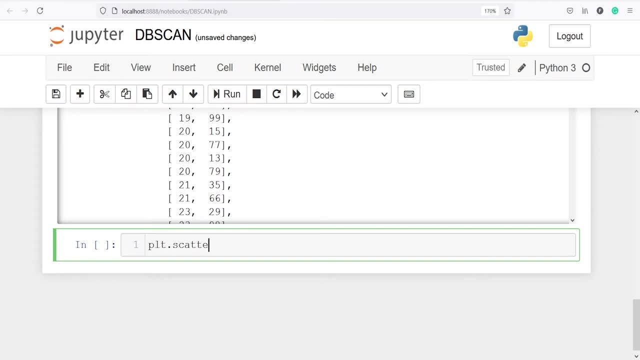 So I will call plt dot scatter, Because I am going to make the scatter plot of these two variables And inside this I will pass a data frame, df, And then I have to pass the index number of these two columns. So the index number of the first one is 0.. 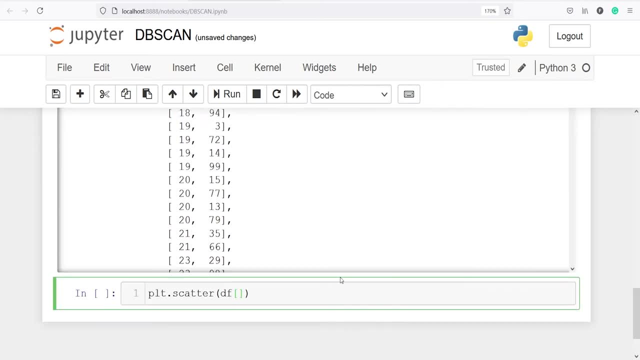 And the index number of the second column is 1.. Here I will write: I want all rows And then the first column. The index number is 0.. Then I will put a comma: df. Now I want all rows And the second column. 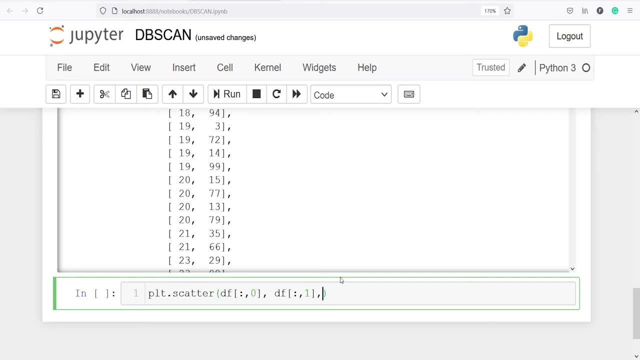 The index number is 1. And I will pass one parameter. s is equal to 10.. This is the size of the dots that you will see in the scatter plot. The next parameter is color, So I will write c, And I want to make it of black color. 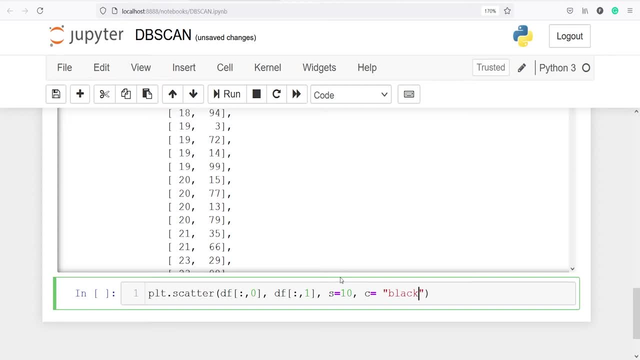 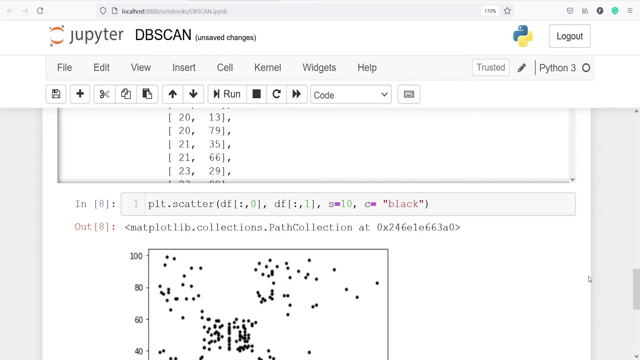 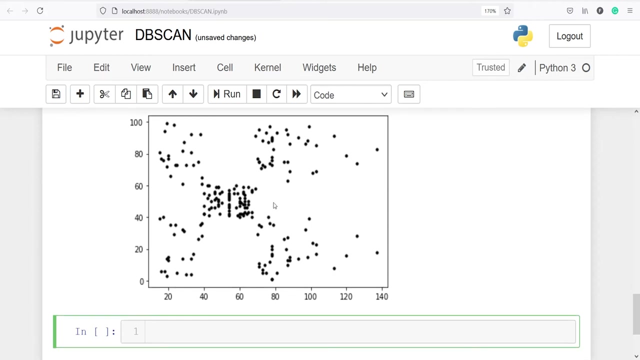 So I will write black here. Let's execute our code And you will see a plot will be coming And here the plot is You can see. So this is a scatter plot And you can see that we can see there are 5 clusters. 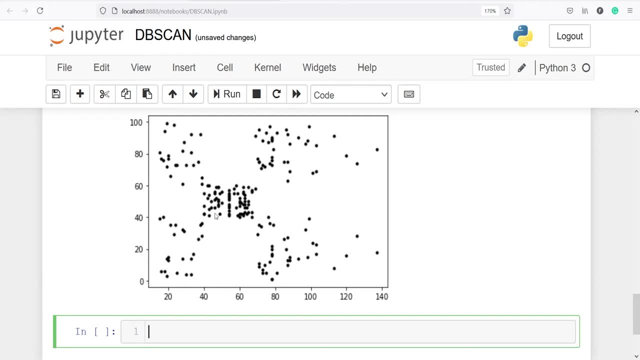 1, 2,, 3,, 4 and 5.. Here are some dots, But these are not forming clusters. They are very far from each other. But if you look at these dots You can clearly see that We can see there are 5 clusters here. 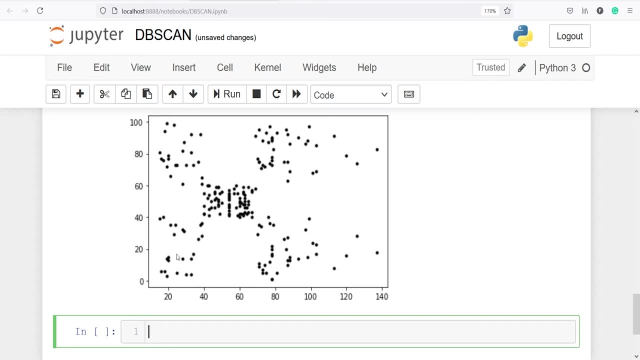 The first one, Second, Third, Fourth And fixed Fifth. So next we will find the optimal number of clusters Using the ELBO method. And using the ELBO method we can actually find the optimal number of clusters. We will use K-means algorithm to perform the ELBO method. 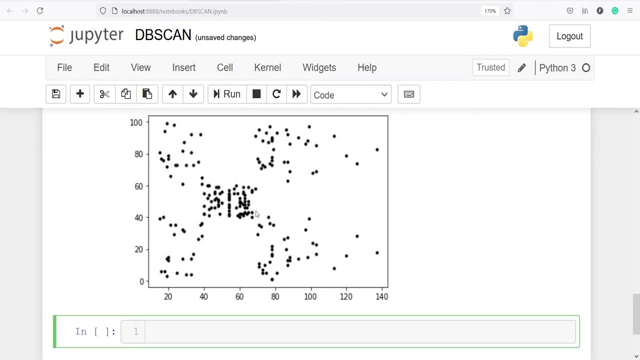 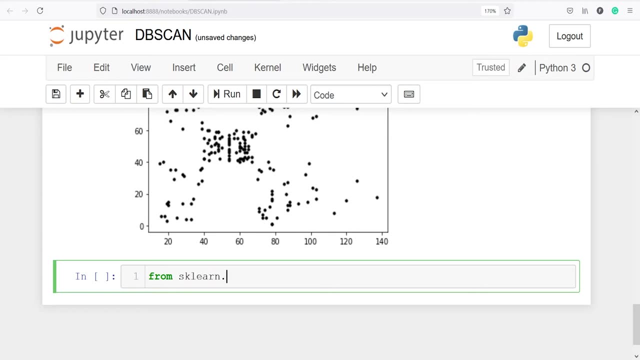 Then we will apply the dbScan algorithm. So for ELBO method We will call this K-means. I will write From sklearnclusterimport K-means. This will help us to use the ELBO method To find the optimal number of clusters. 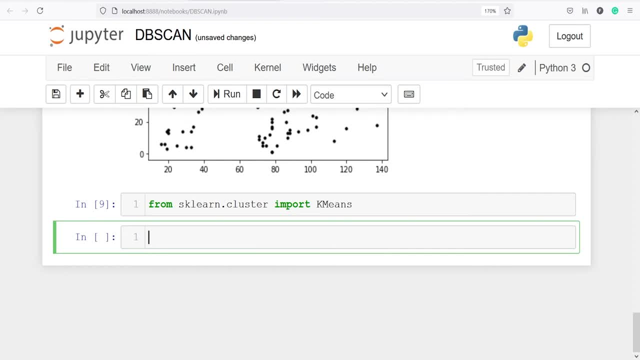 Let's execute our code. So we have imported this K-means. Now I will make one variable WCSK. So this is within sum of cluster scores. This is going to be an empty list. I am going to save the result in this empty list. 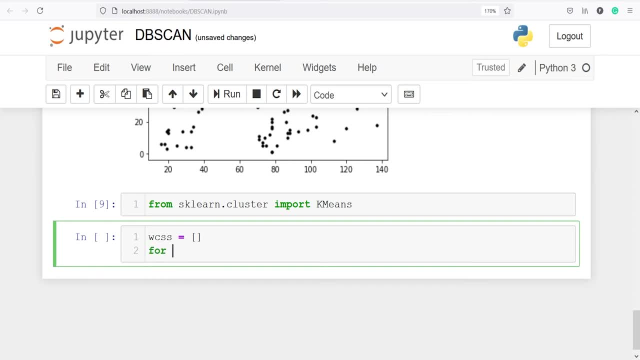 Then I will run a for loop For i in range 1 to 11.. I want to run it 10 times. That's why I have put 11 here, Because it will exclude the last number. The last number is 11.. 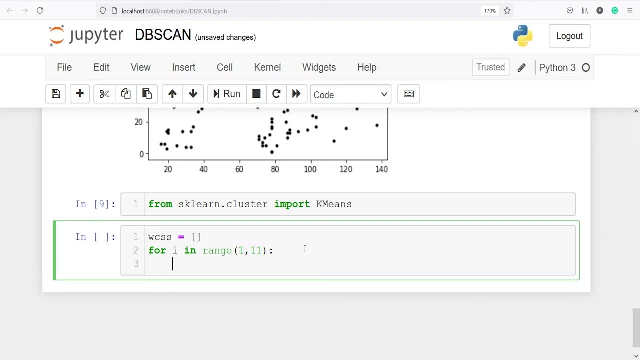 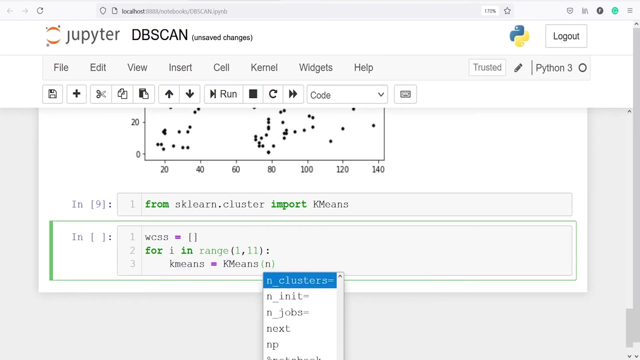 It will only run up to 10.. Then I will make One variable, K-means. Now from K-means, I will call this method K-means And inside this I will pass one parameter And cluster. That is the number of clusters we want. 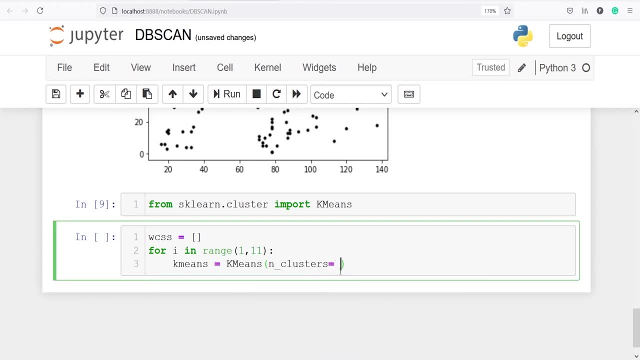 So I will put here i, Because we are running a for loop And in i we will have 10 values, starting from 1 to 10.. That's why I am putting this i here, So our number of clusters is going to be 10.. 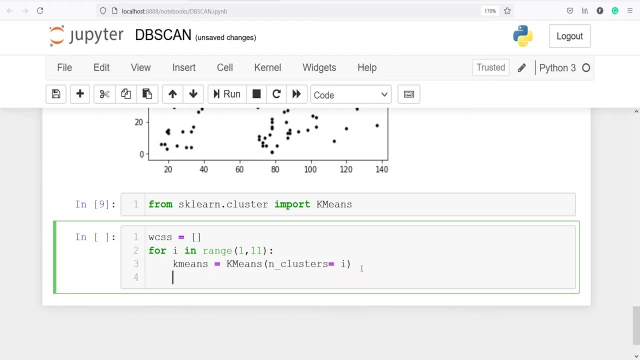 Next, I will make one variable innate And this will have the method. So I will type K-means here, K-means plus plus. This will calculate the distance from the center. Then the next parameter is maximum underscore iter, And this is going to be 300. 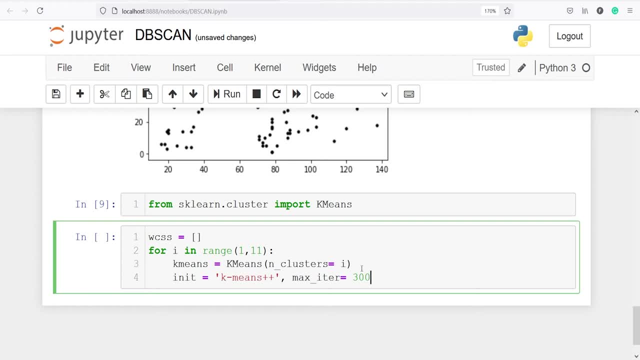 So here I am saying that This will run maximum. the number of times is 300.. It will not run beyond 300.. I will put one comma here. I will just have to remove this bracket And I have to put comma here. 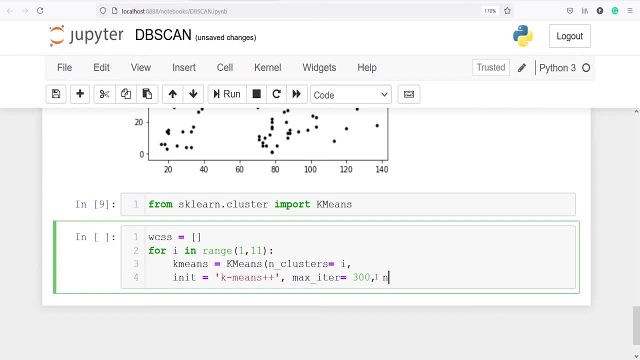 Then the next parameter is N-innate, And this is going to be 10.. Now we will fit the K-means. So we will call K-means dot fit And we are going to fit it on the data frame DF. 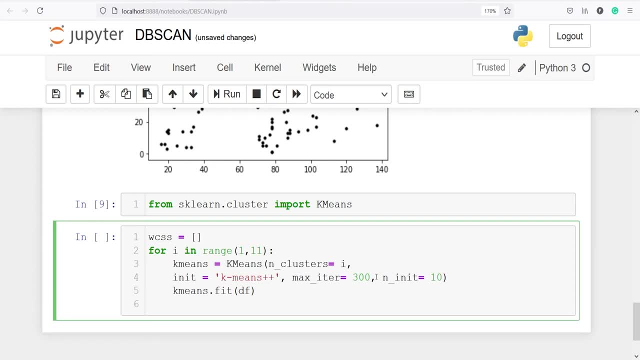 Then we will come out of the loop And we will start this plot, PLT, dot plot Range from 1 to 11. And we will put WCSS. So this 1 to 11 will be on the x-axis And these numbers will be on the y-axis. 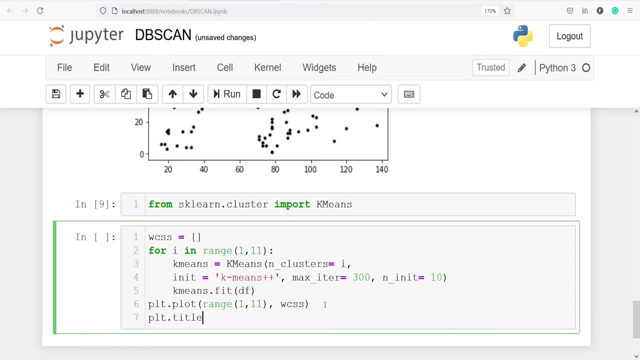 Then PLT dot title, And the title will be the ELBO method. Then we have x-label, PLT dot, x-label. Our x-label will have number of clusters, So this will show the number of clusters on x-label. And then we have y-label. 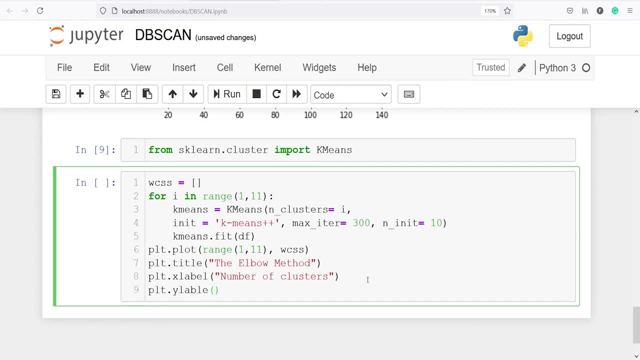 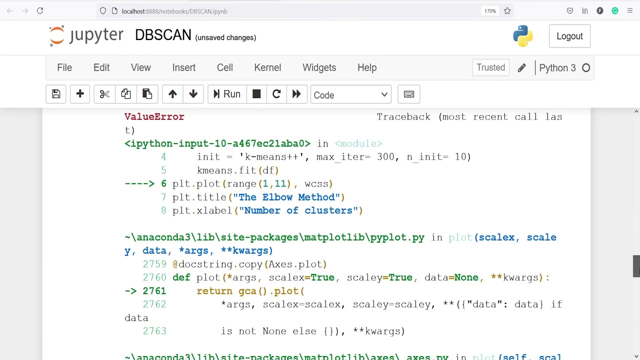 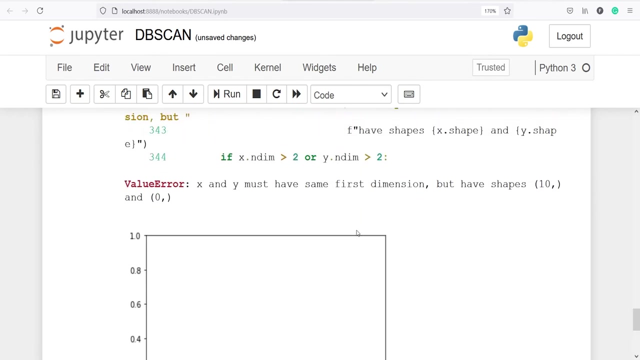 PLT dot y-label. On y-label we will have WCSS score. So these are the within sum of clusters score. Then PLT dot show. Let's execute our code. And we got some error here. I got the error. And here it says x and y must have same first dimension. 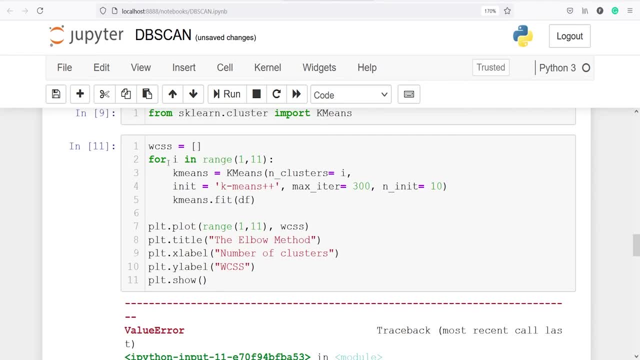 This error is because I forgot to append this Empty list. So I will call this WCSS, This empty list, And then I will append the result. The results are saved in this kmeans dot inertia underscore. Now let's execute our code. 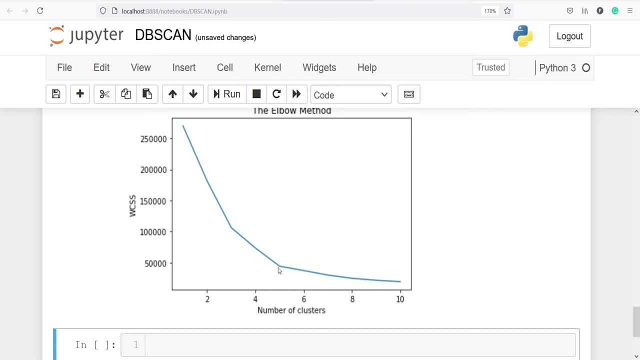 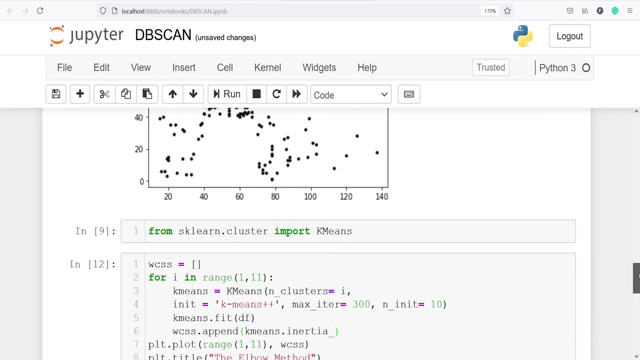 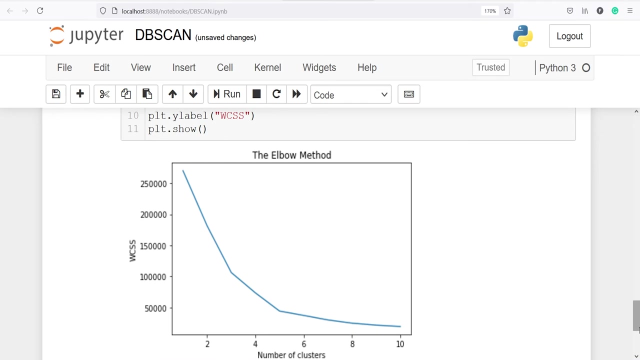 The optimal number of k is at this 5 here. So the number of clusters we are going to make is 5.. And we have already seen here in this scatter plot also That the optimal number of clusters are 5.. And this db scan for the elbow method: 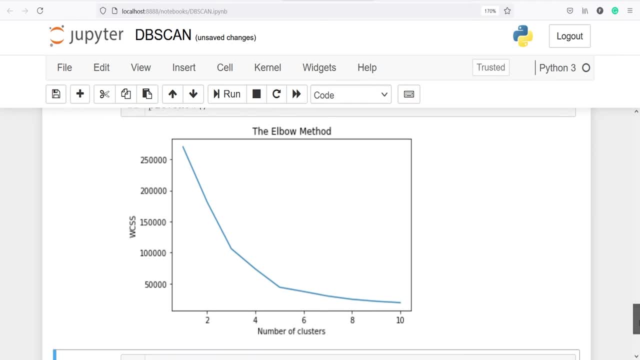 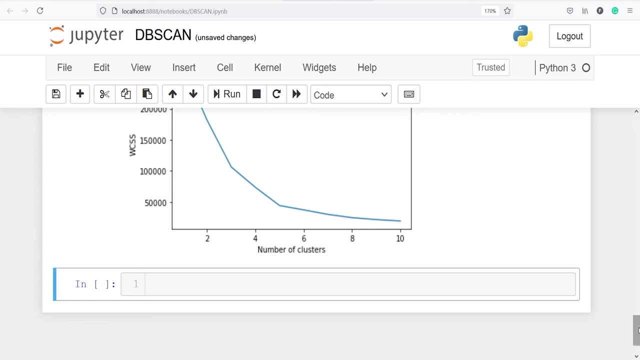 It is also showing that the optimal number of clusters should be 5.. So we are going to go with the 5 one. Next, we will fit the db scan to the data set. So from sklearn dot cluster I will import db scan. 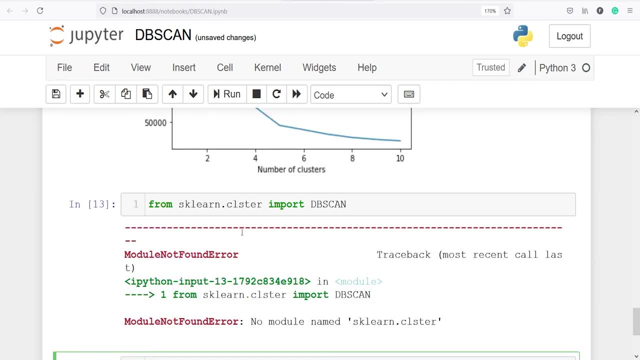 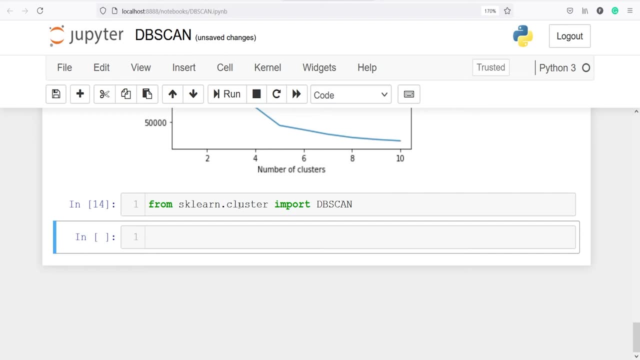 Let's execute our code: sklearn dot cluster. I have to put u here. Let's make an object of db scan With two parameters Or the two default values. So I will make one variable, db scan. Then I will call the class. 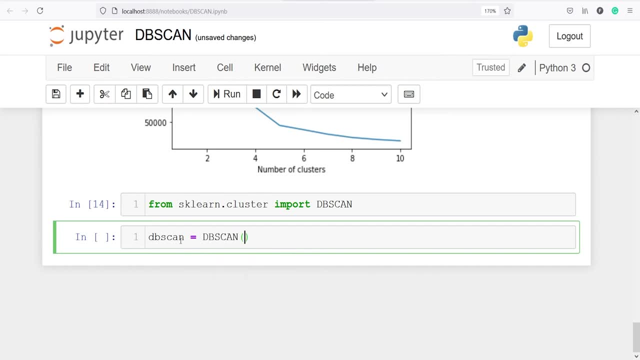 db scan And in this I will pass two parameters: The epsilon and the minimum points There. So I will type eps- It is going to be 5.. And the minimum number of samples. So minimum number of samples we are going to take as 5.. 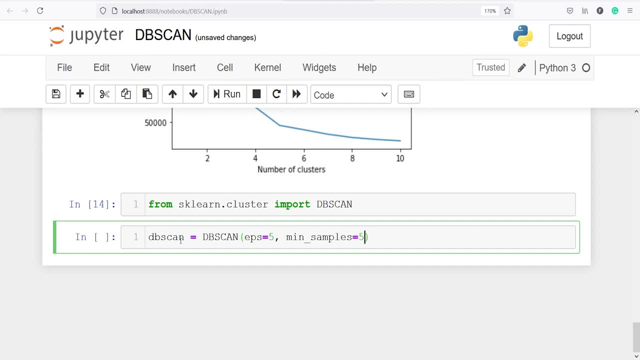 Here epsilon means that it is the first radius Within which we want to examine the number of objects, And the minimum samples here represent that Minimum number of samples that need to be present inside the circle With the minimum radius of epsilon. Minimum radius of epsilon. 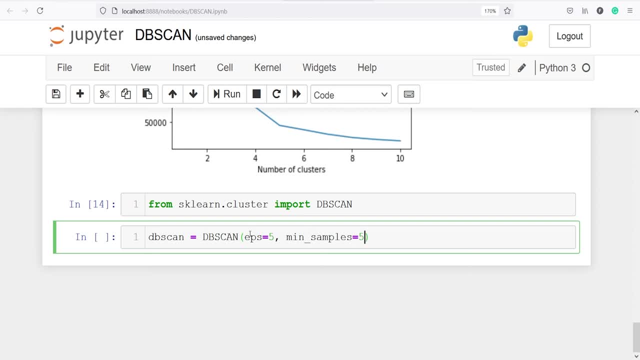 So this- both minimum samples and epsilon- are connected to each other. Let's execute our code. So we have created the clusters And to check the number of clusters We will make a variable unique And save the total number of clusters in that. 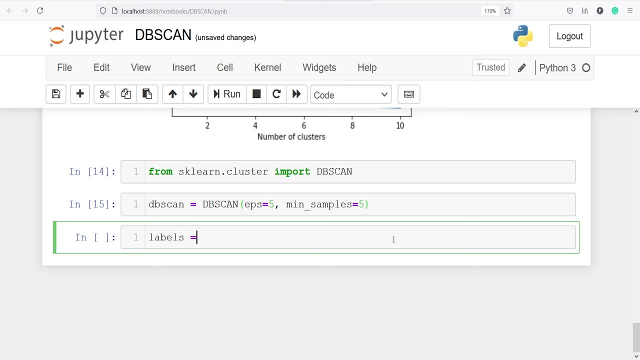 So I will make one variable Labels And then I will call db scan From this. I will call the method fit, underscore predict, And then I will pass the parameter df. And now I will call the unique method from numpy To check the number of clusters. 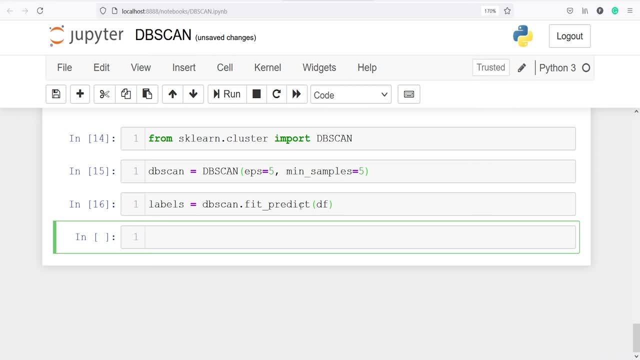 So using this fit predict, we have saved the number of clusters that are required In this variable labels And to check those numbers We will use the numpy From numpy. we will call unique This unique method And labels. We will pass the variable labels here. 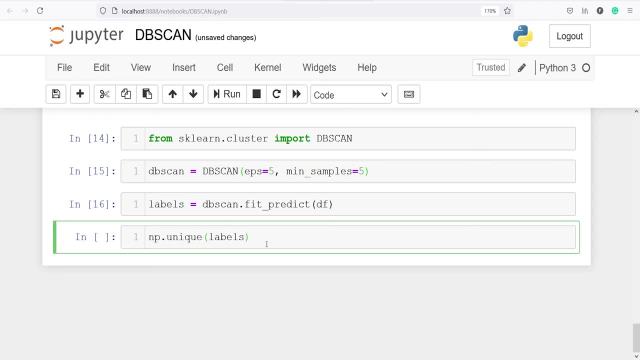 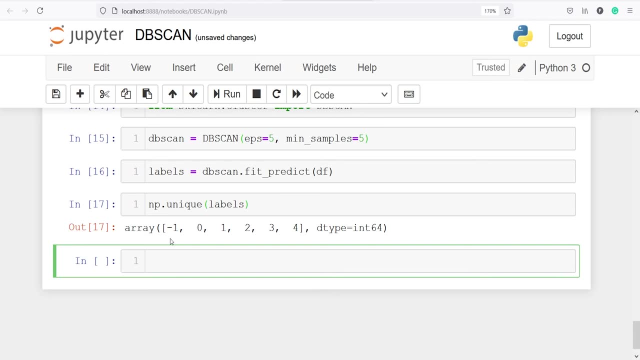 That we have saved above. Let's execute our code. So we got minus one, Zero, One, Two, Three And four. So these are the clusters that we got Here. you will find that we got minus one, But this is not a cluster. 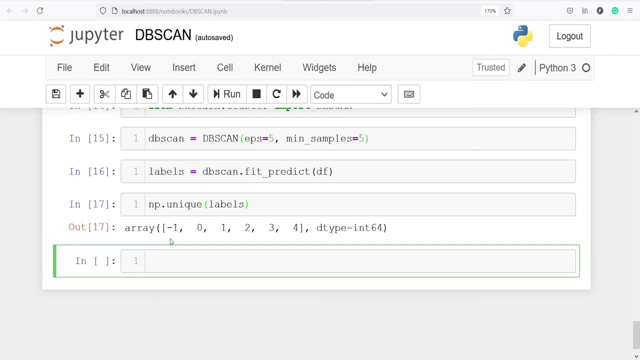 db scan labels noises as minus one. So it got noise in the data set And it labels that noise as minus one. So minus one is not a cluster but a noise. But if the algorithm does not find noise in the data set, Then minus one will not be present in the unique labels. 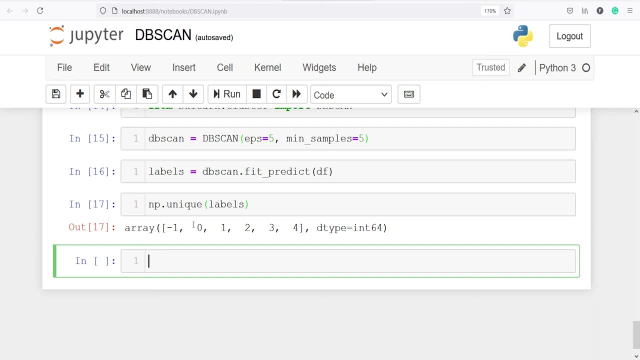 So do not worry if you do not get minus one on your data set. In this data set you will definitely get minus one, But when you are working on some other data set Or you download it from somewhere else And you try to apply the db scan algorithm, 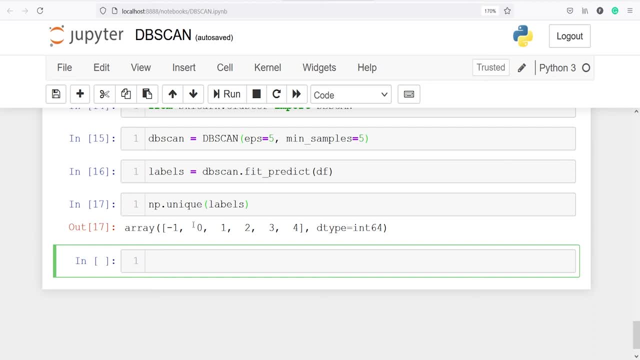 And there you see that you did not get minus one. So in that case, do not get worried about that, Because you will get minus one only If you have, If there are any noise present in the data set. Now let's visualize our cluster. 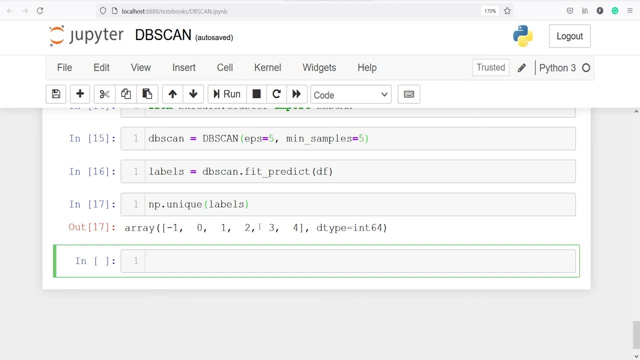 So we have total five clusters: Zero, One, Two, Three And four. Now we are going to visualize these clusters And we will use the matplotlib library. I will call pltscatter, Then I will call the data frame df, Then from this I will call the method ilac. 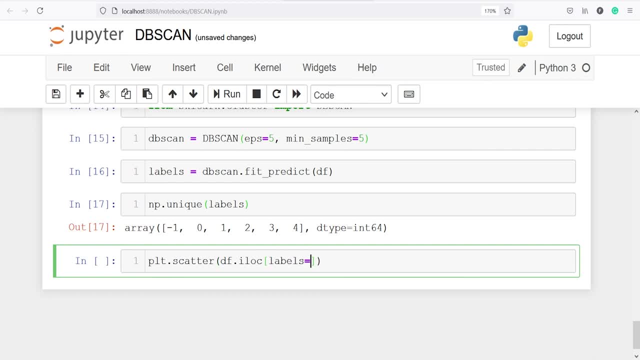 And then labels is equal to minus one And zero, Then df of labels is equal to Minus one And one. Then we will pass the parameter. S is equal to twenty. Color is going to be black Or you can take any color here. 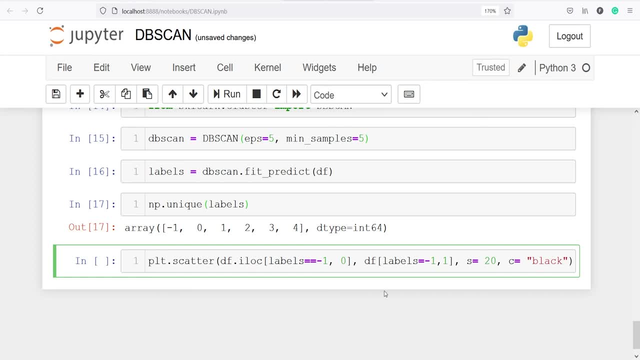 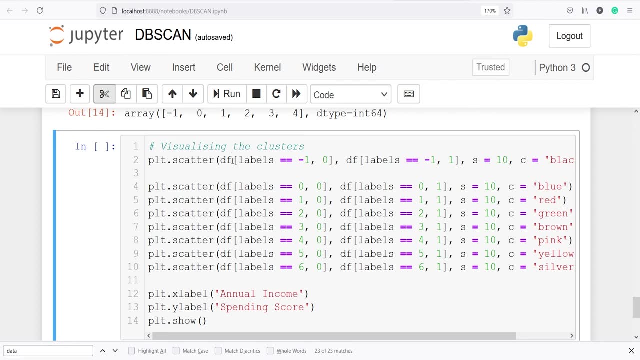 And we will repeat this five times Because there are five clusters. For saving time, I have copied and pasted all the codes here. I have removed that ilac from here Because we don't need the ilac here, So you have to do this. 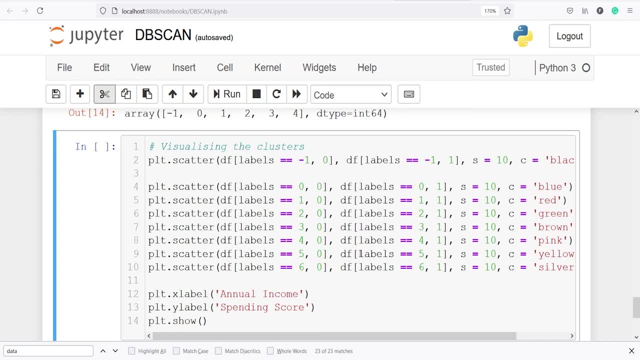 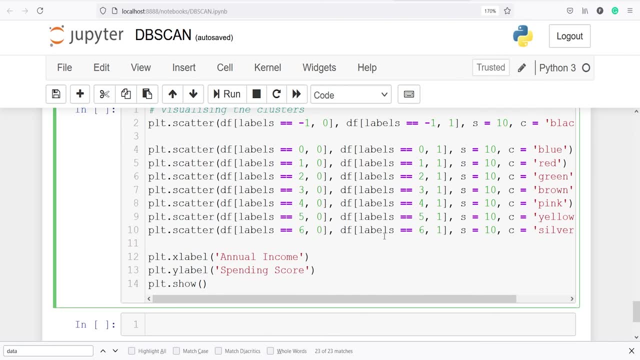 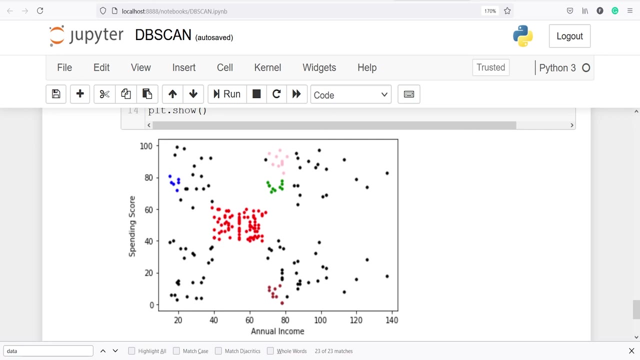 You have to put all the cluster numbers here. I will provide you with the jupyter notebook. You don't have to worry about that Now. let's execute our code Now. here you will see. we got the results here, So the red cluster is identified correctly. 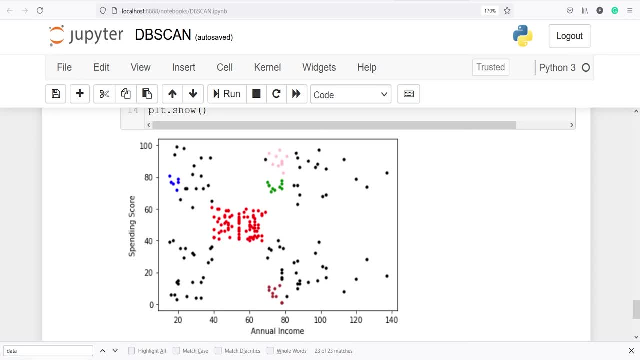 DBSCAN looks for the density around the point And in our red cluster we see points are dense, But at the places, At the different places, The points are not dense, But they are all scattered all over. You will see here, Even in blue. 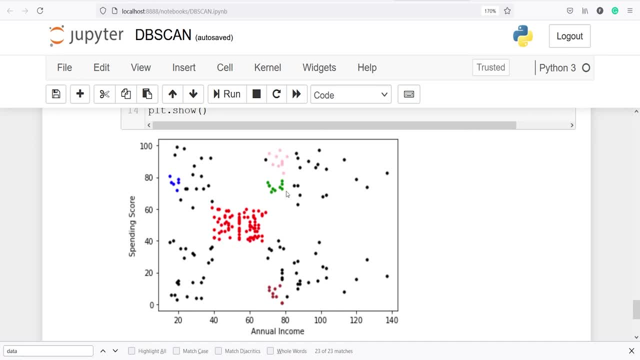 Green, Here you will see, the points are not very much dense, They are almost scattered. We have a very less number of points which are dense here. Even in blue- here we will see- Five to six points are dense, But most of the points are scattered all over. 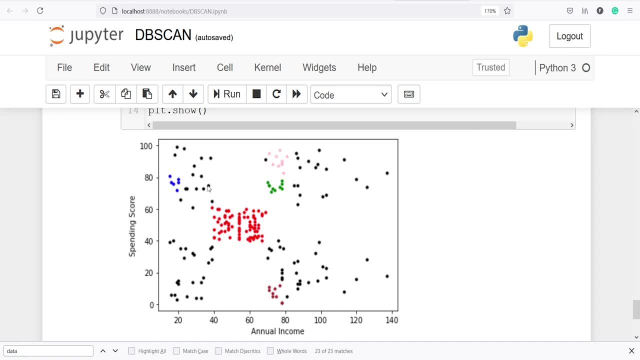 Because black dots are less dense than the red dots. You will see, The red dots are very, very dense. They are very close to each other And these black dots are very far away from each other. So because black dots are less dense than the red dots, 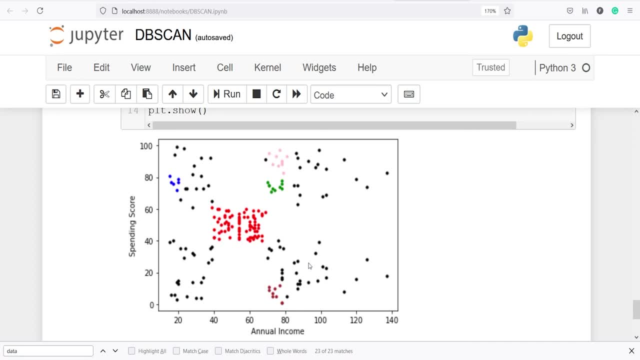 They are considered as noise in the data set. The idea in the DBSCAN is that The objects belonging to a certain cluster Should be denser compared to its surrounding. We can see that red dots are denser than the other dots, And so DBSCAN has found this cluster correctly.